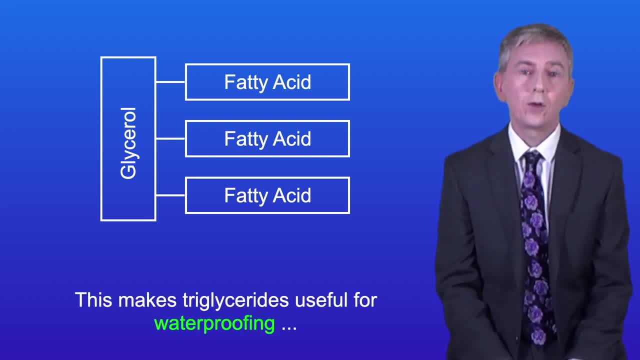 they will not dissolve in water. This makes triglycerides useful for waterproofing, and we saw that in the previous video. Now, phospholipids have a structure which is similar to triglycerides, but different in one key way, And this difference has a major effect on the way that phospholipids 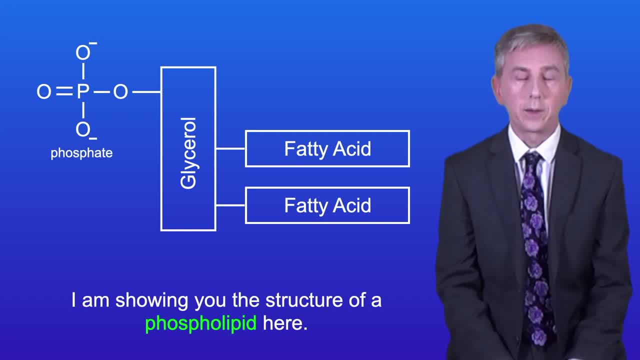 behave. I'm showing you the structure of a phospholipid here. As you can see, a phospholipid has a glycerol molecule bonded to two fatty acid molecules. The glycerol molecule is also bonded to phosphate. Now phosphate looks complicated, but you don't have to learn the structure. 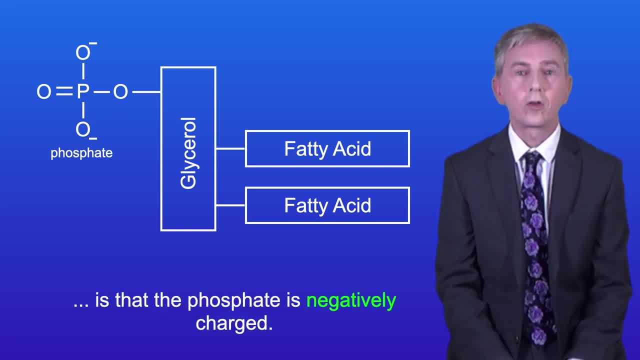 The key idea that you need to get is that the phosphate is negatively charged, In other words, this part of the molecule is polar. Because of this, the phosphate group is hydrophilic, In other words, it attracts water molecules. Now I should just point out that, in reality, phospholipid molecules are slightly more complicated. 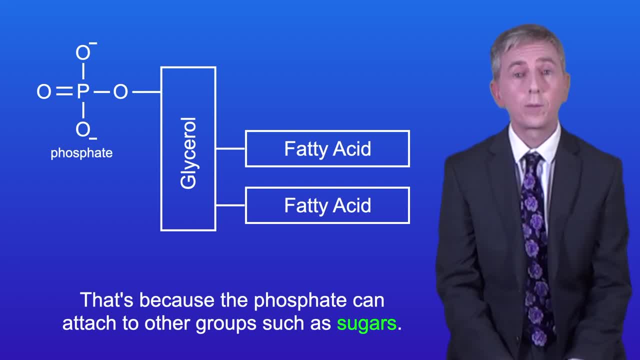 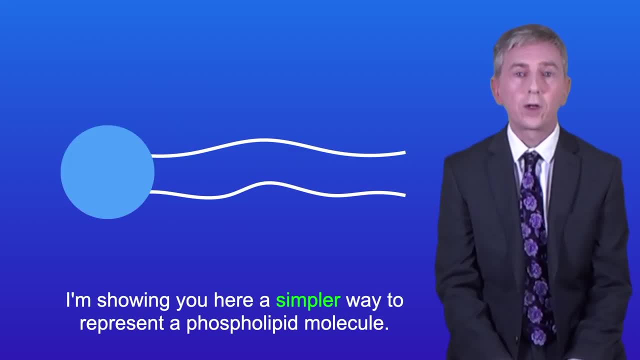 than this, And that's because the phosphate can attach to other groups, such as sugars. We look at that in more detail in later topics. I'm showing you here a simpler way to represent a phospholipid molecule, In this case the. 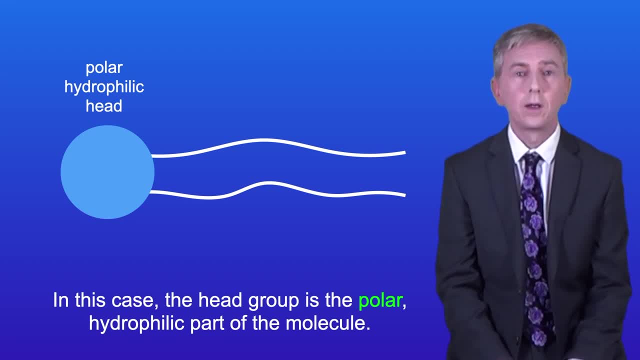 head group is the polar, hydrophilic part of the molecule. The tails represent the two fatty acid molecules, And remember that these are non-polar and hydrophobic. So, as you can see, phospholipids contain both a hydrophilic and a hydrophobic region. This means that 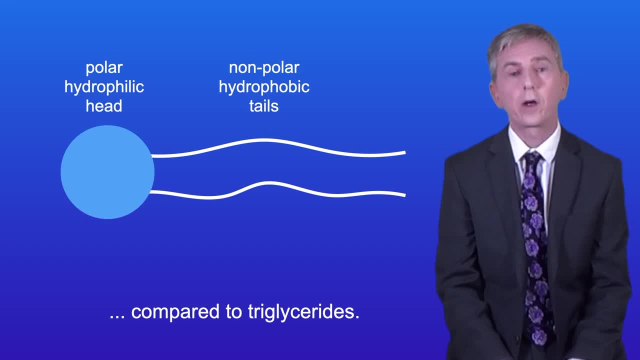 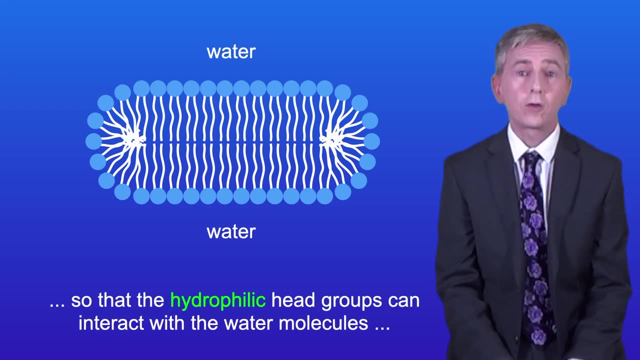 phospholipids behave very differently in water compared to triglycerides. In water, phospholipid molecules position themselves so that the hydrophilic head groups can interact with the water molecules, while the hydrophobic tails cluster together well away from water molecules. 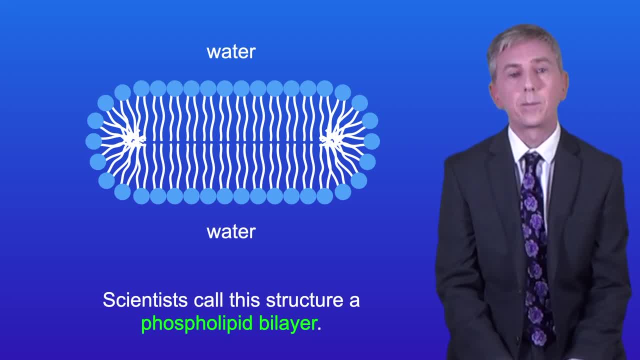 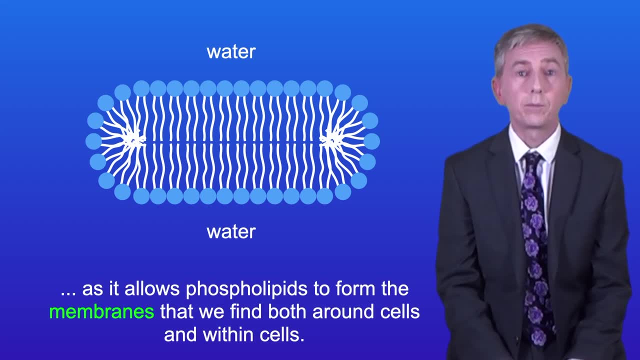 Scientists call this structure a phospholipid bilayer. Now this property of phospholipids is extremely useful, as it allows phospholipids to form the membranes that we find both around cells and within cells. You'll be seeing this again when we look at cell membranes in more. 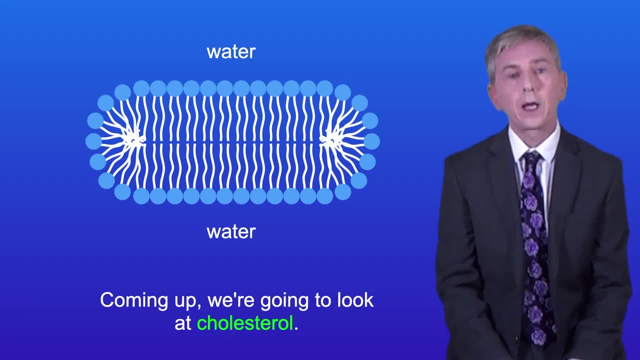 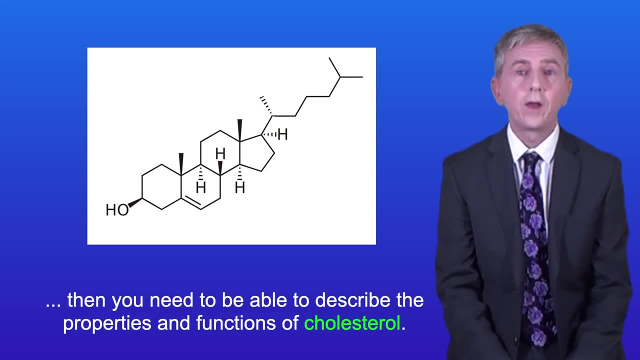 detail in later videos Coming up. we're going to look at cholesterol. OK, now, if you're following the OCR spec, then you need to be able to describe the properties and functions of cholesterol. Cholesterol is part of a family of lipids called sterols. As you can see, cholesterol